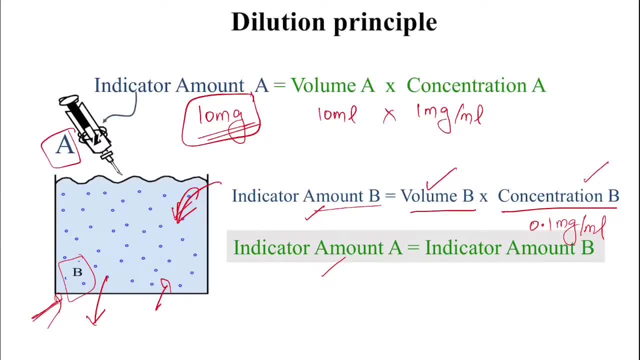 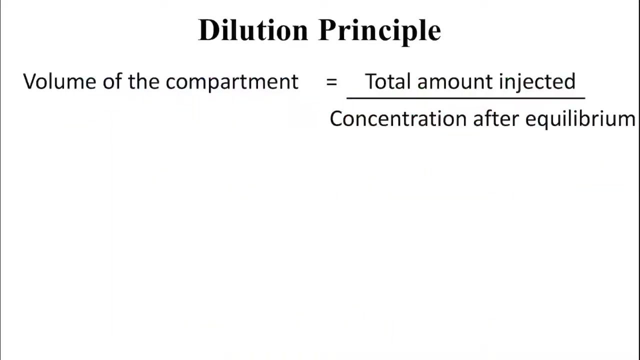 remains within this compartment B. If we rewrite this we don't know only this volume B. So volume is going to be 100 ml. So this is the volume of this compartment. So this is the broad principle which we are going to use for measuring all the compartment volumes. Only thing we have to be sure: 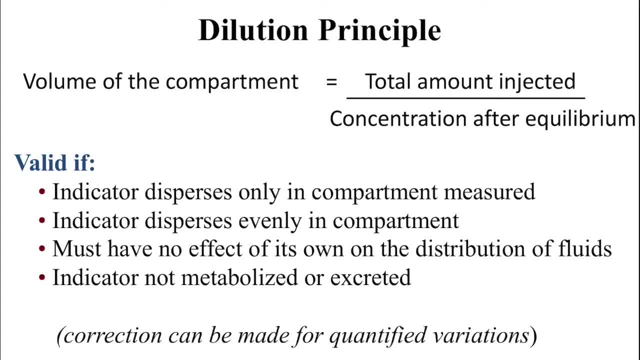 is that the characteristics of the dye which we are choosing should stay only in the compartment we intend to measure. So this is the volume of this compartment. So this is the volume of this compartment. If you want to measure the extracellular fluid volume, then the dye we 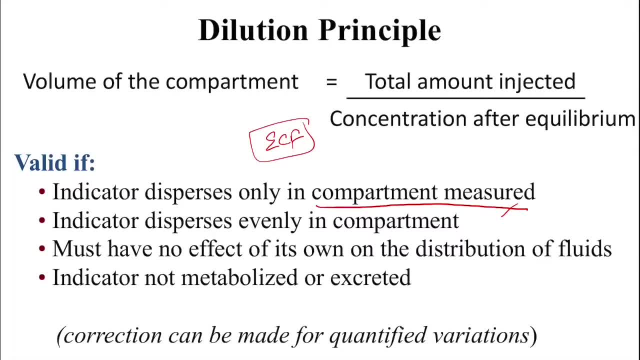 inject should stay only in the extracellular fluid and should not enter the cell, And it should disperse evenly within the compartment It should not stay within. for example, it should not stay more in the interstitial fluid and less in the plasma within ECF. Then we are going to have a 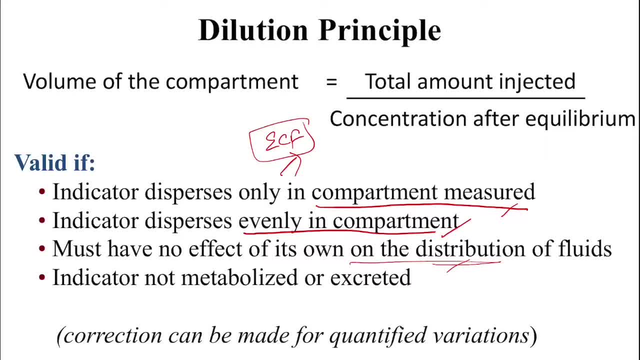 wrong value. It should not have any effects on its own on the distribution of fluids and it should not be metabolized or excreted. during the period in which we are estimating, We may not get a dye which absolutely satisfies all the requirements of the compartment. So this is the volume of the 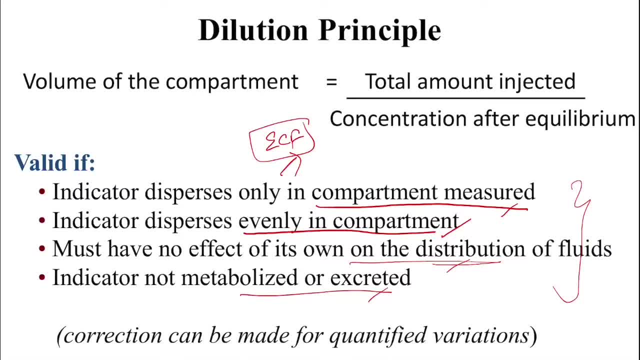 compartment. So this is the volume of the compartment. So this is the volume of the compartment. So sometimes if some known amount of dye is getting excreted, we might have to do correction for that in our calculations. Let's start with plasma. Here we use a dye called Evans blue. because Evans blue 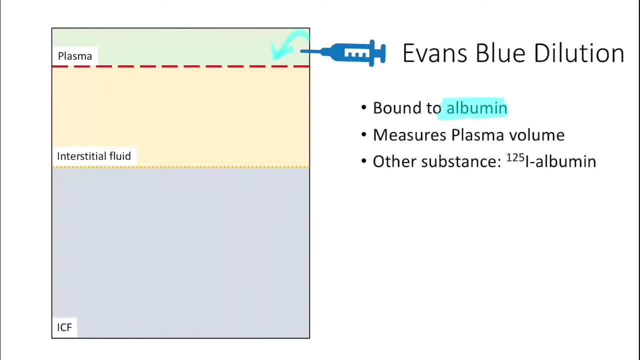 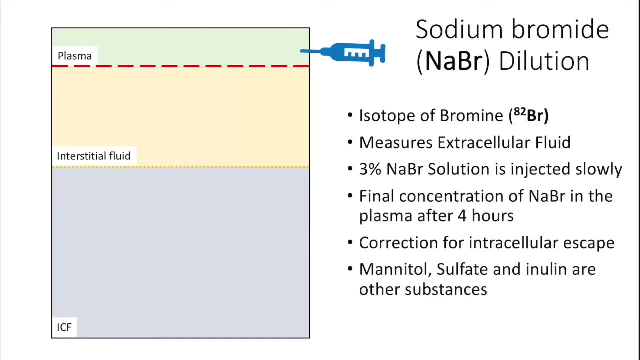 is tightly bound to albumin. Once injected into this compartment it stays only within the plasma. So when we take the final concentration it gives the estimate of plasma volume. The other substance is the iodine label albumin sodium bromide. here it has an isotope of bromine, radioactive isotope 82. 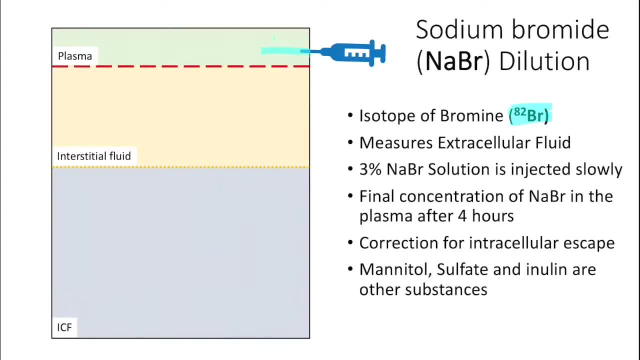 bromine. once the bromine is injected into the plasma it goes actually into the interstitial fluid also, so the entire extracellular fluid compartment as filled with bromine. so if we take a final value from this compartment, it's going to estimate extracellular fluid volume. 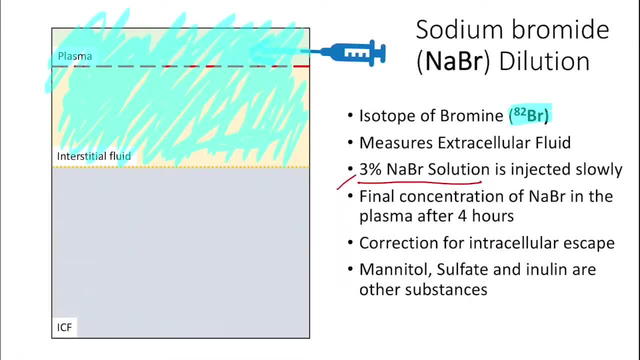 we inject about three percent of sodium bromide solution slowly and we measure the final concentration after four hours and some amount of bromine also escaped, is into the intracellular fluid and we have to make correction for that. these are the other substances used in the measurement of extracellular fluid volume. deuterium oxide: it is a isotope of hydrogen. 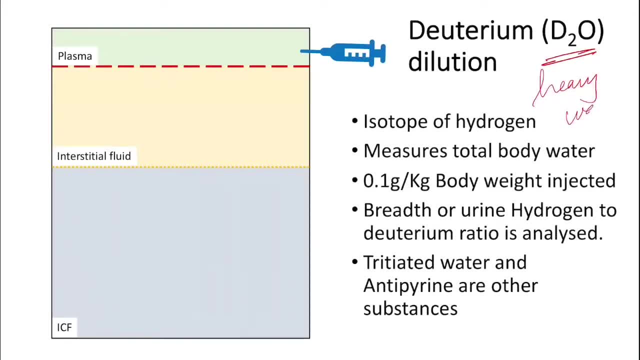 when it is present along with oxygen, we call it as heavy water, and when this is injected it behaves like this and it is injected into the extracellular fluid volume, so it goes into all the compartment, so everywhere, all three compartments it equally distributes. so we inject around 0.1 per kg of body weight. we measure the final concentration using either: 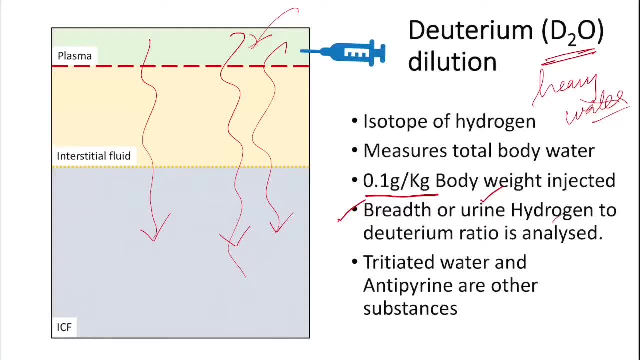 breath or in the urine sample. we can measure hydrogen to deuterium ratio and we can calculate the whole body sample and deuterium is not a radioactive so it is safe to use in smaller quantities. and the other isotope of hydrogen is the tritiated water, which is actually radioactive. 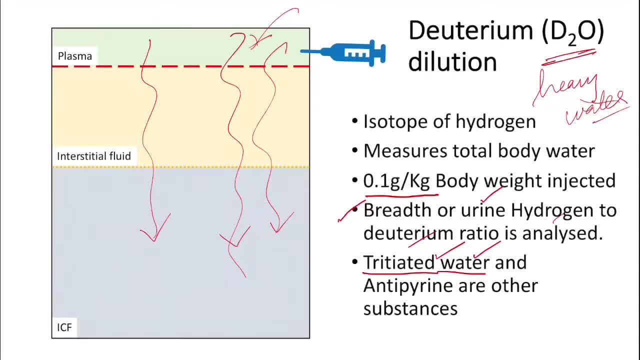 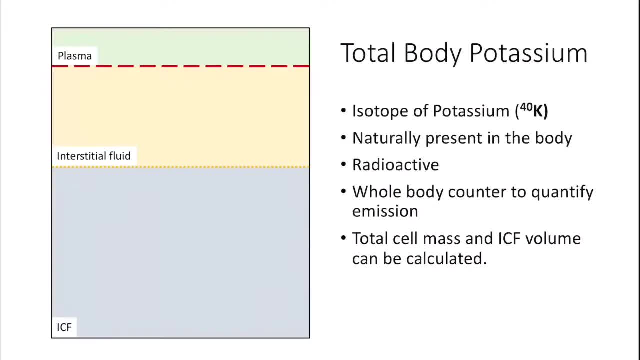 it is not safe. it was once used to calculate the volume of total body water. the other substance is antipyrene for total body water estimation, total body potassium. this is different from other estimation so far we have seen, because we don't have to inject anything. this is naturally. 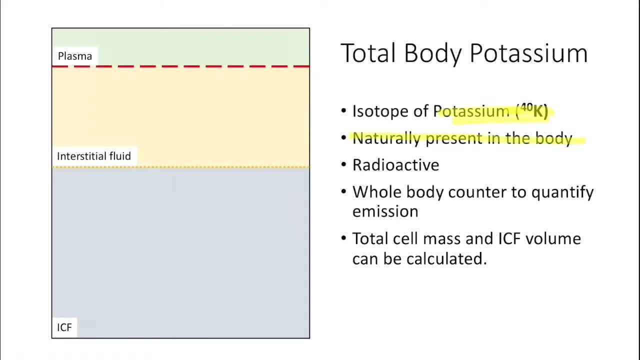 present in the body. this is radioactive isotope of potassium and we are going to use a whole body counter to quantify the emissions from this potassium: total cell mass, intracellular fluid volume or the certain things we can calculate using the total body potassium estimation. the next method we are going to see is the bioimpedance analysis. this is non-invasive. 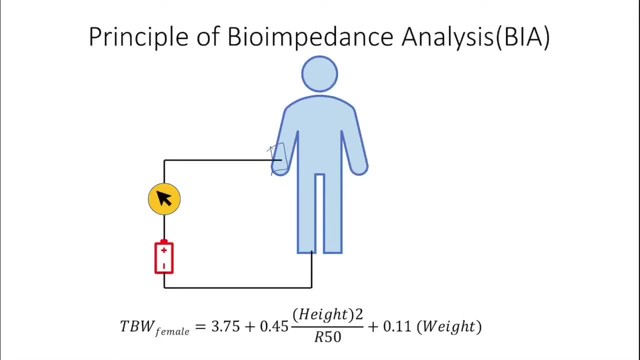 procedure here we are going to inject current at two different points in the body, a known quantity of current, and we are going to measure how much is the current flows across so effectively. we are going to measure the resistance or the impedance for the flow of current and after measuring this resistance- r50 stands for measuring at 50 hertz- we are going to use